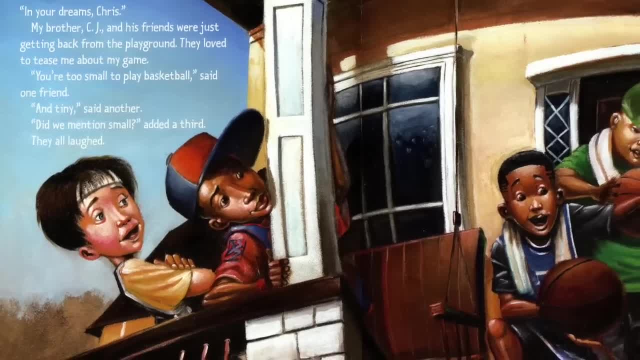 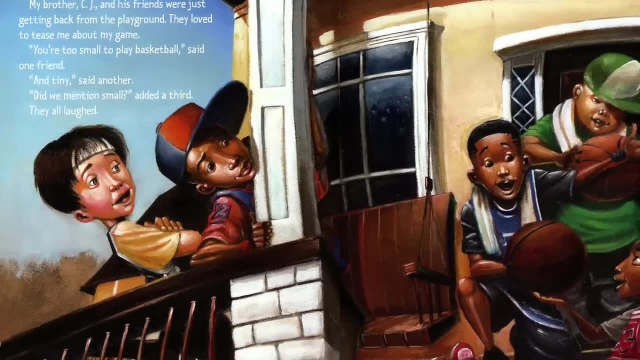 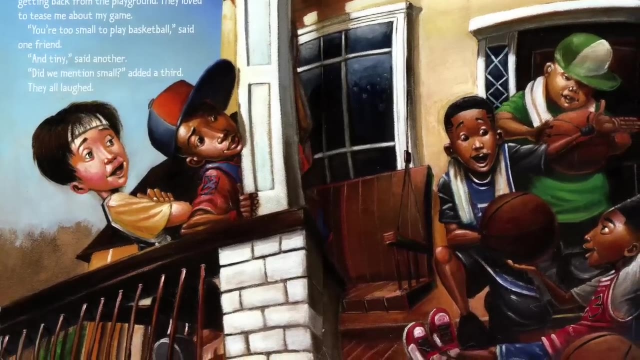 My brother, CJ, and his friends were just getting back from the playground. They loved to tease me about my game. You're too small to play basketball, said one friend, And tiny, said another. Did we mention small? Added a third. They all laughed. 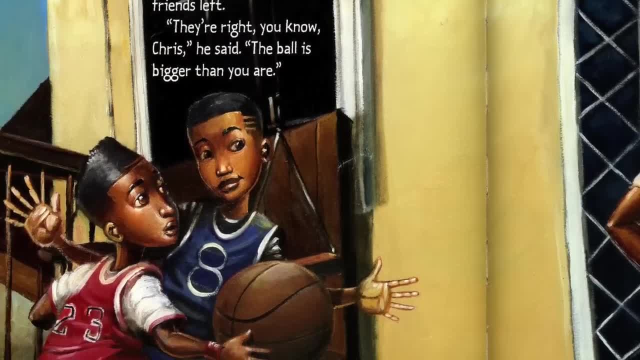 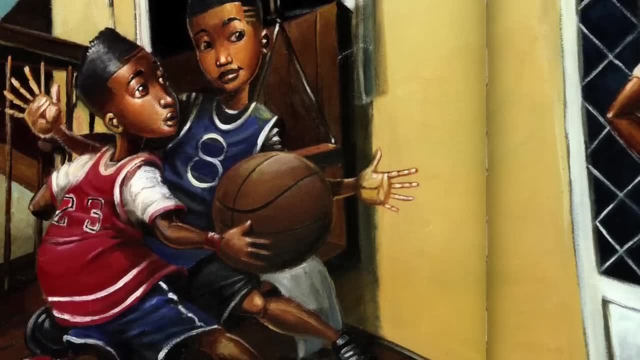 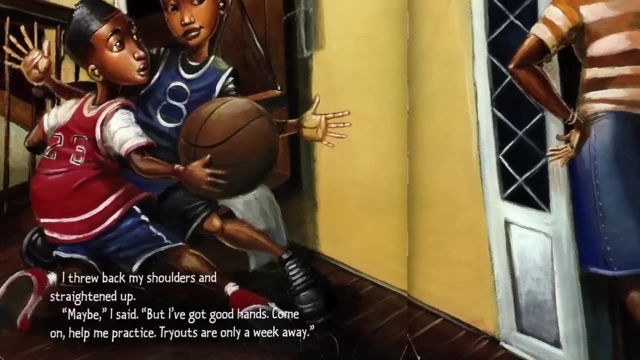 CJ stayed behind as his friends left. They're right, you know, Chris. he said: The ball is bigger than you are. I threw back my shoulders and straightened up Maybe. I said: But I've got good hands, Come on, help me practice. 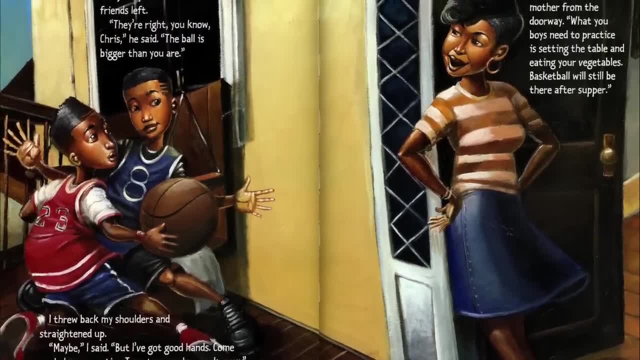 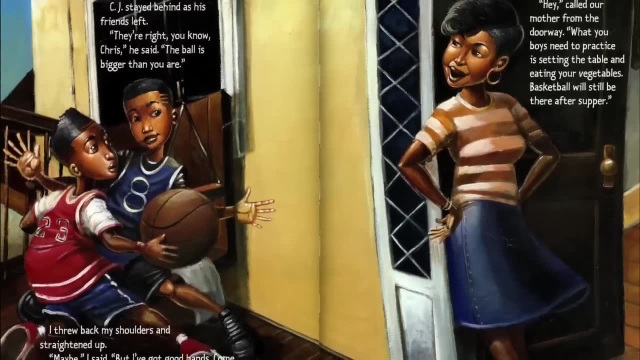 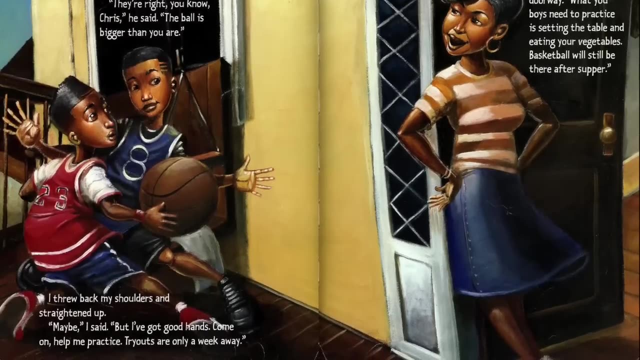 Tryouts are only a week away. Hey called our mother from the doorway. What you boys need to practice is setting the table and eating your vegetables. Basketball will still be there after supper, But we're still going to have to get to the game and get to our game. 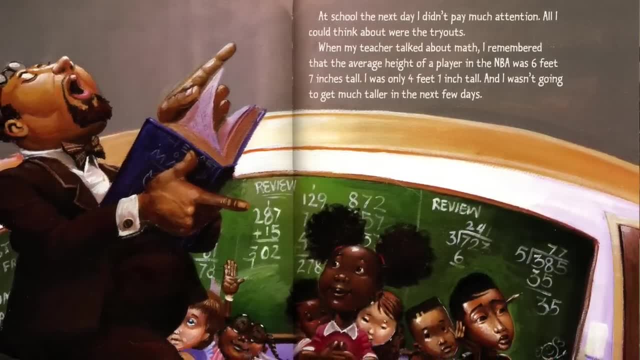 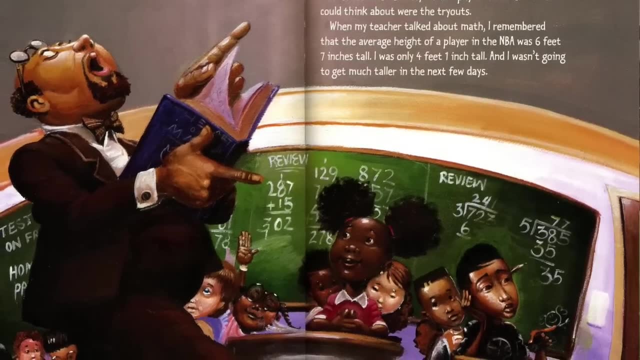 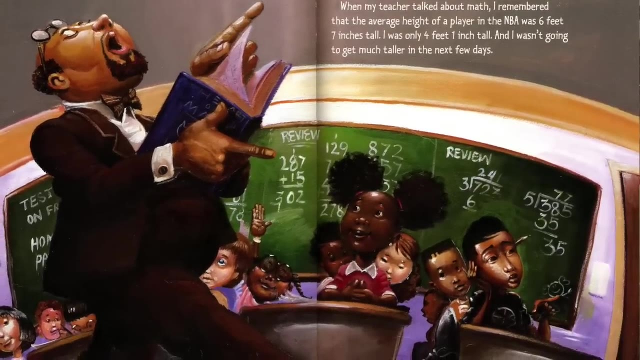 At school the next day I didn't pay much attention. All I could think about were the tryouts. When my teacher talked about math, I remembered that the average height of a player in the NBA was six feet seven inches tall. I was only four feet one inch tall and I wasn't going to get much taller in the next. 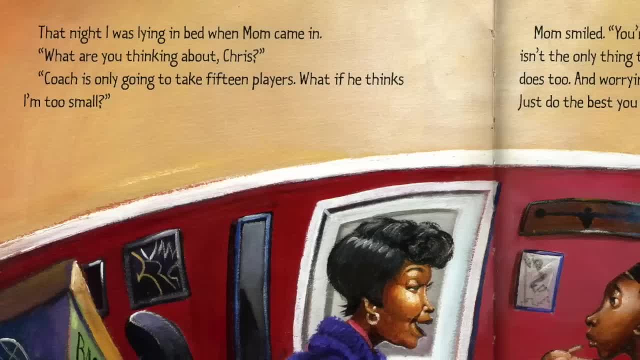 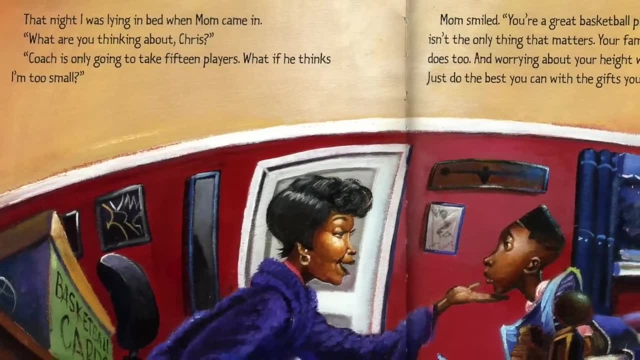 few days. That night I was lying in bed when Mom came in. That night I was lying in bed when Mom came in. What are you thinking about? Chris Coach is only going to take 15 players. What if he thinks I'm too small? 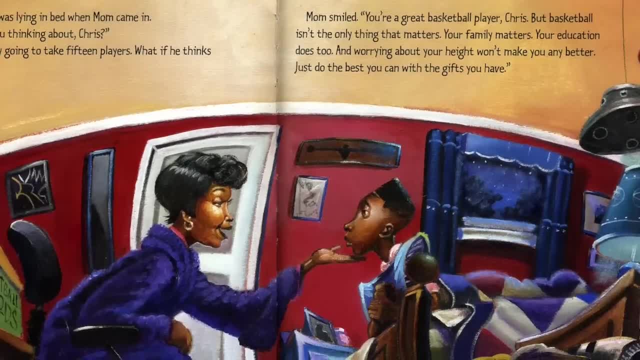 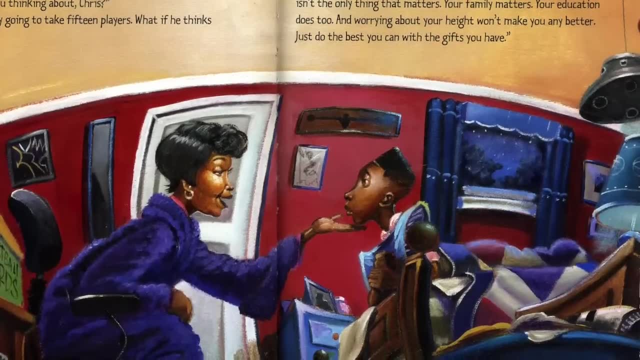 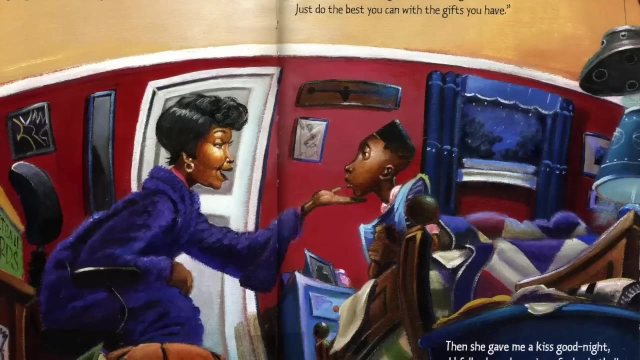 Mom smiled. You're a great basketball player, Chris, But basketball isn't the only thing that matters. Your family matters, Your education does too, And worrying about the height won't make you any better. Just do the best you can with the gifts you have. 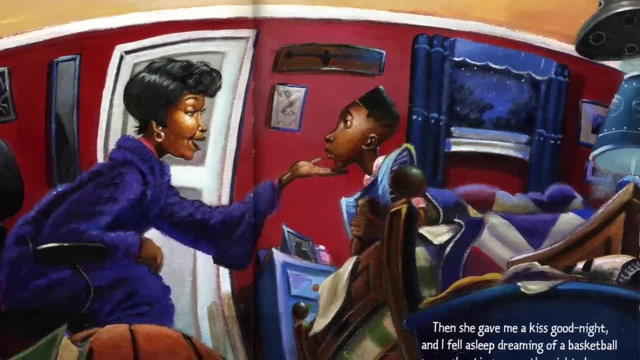 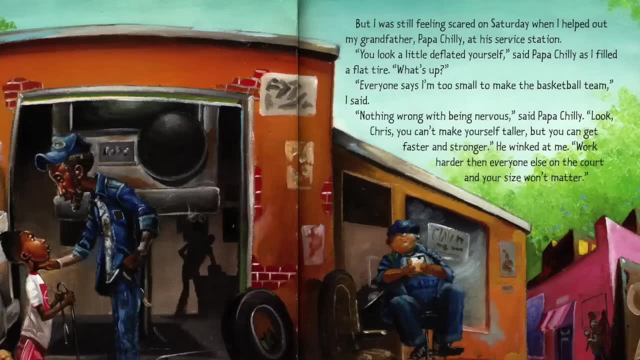 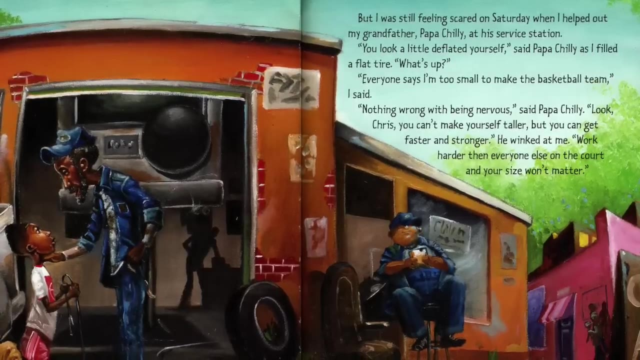 Then she gave me a kiss goodnight and I fell asleep dreaming of a basketball moon shooting across the night sky. But I was still feeling scared on Saturday when I helped out my grandfather, Papa Chili, at his service station. You look a little deflated yourself. 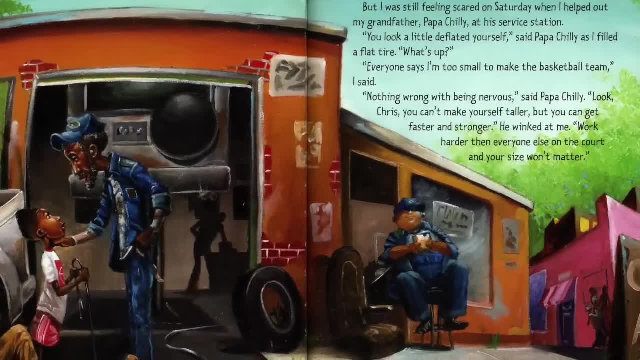 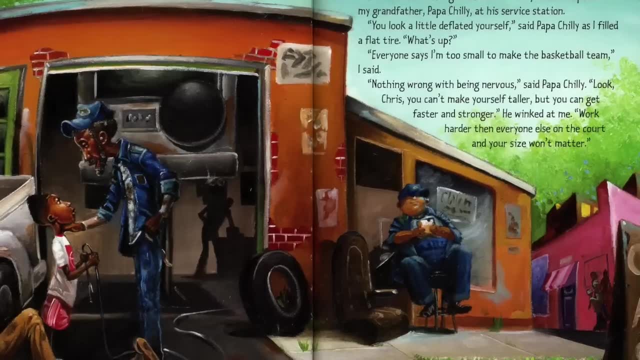 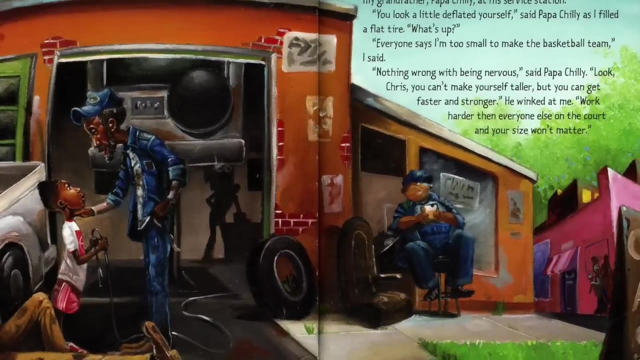 said Papa Chili, as I filled a flat tire, What's up? Everyone says I'm too small to make the basketball team. I said Nothing wrong with being nervous, said Papa Chili. Look, Chris, you can't make yourself taller, But you can get faster and stronger. he winked at me. 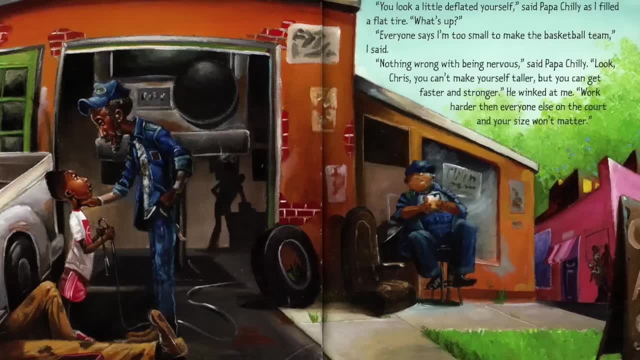 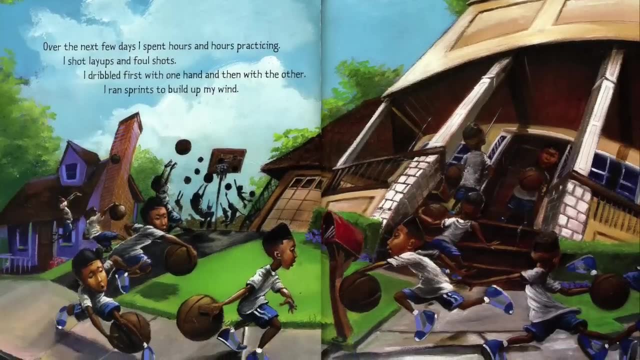 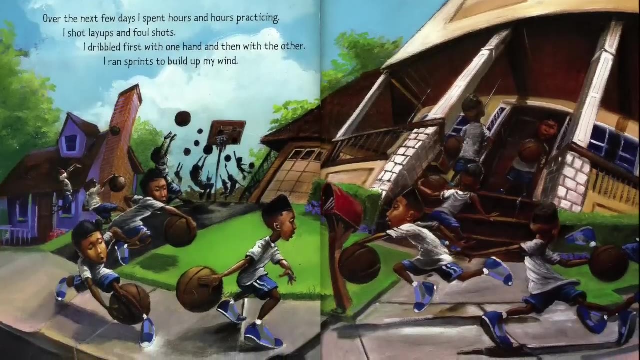 Work harder than everyone else on the court, and your size won't matter. Over the next few days, I spent hours and hours on the basketball court. I spent hours practicing. I shot layups and foul shots. I dribbled first with one hand and then with the other. 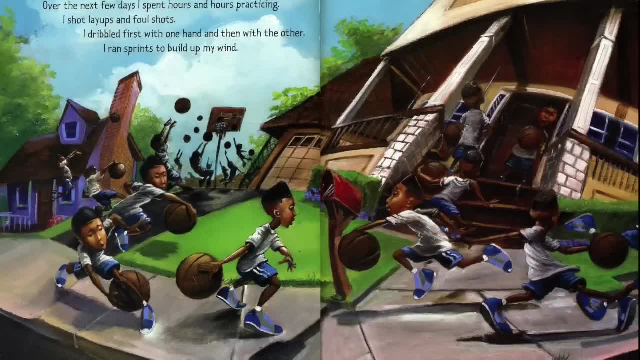 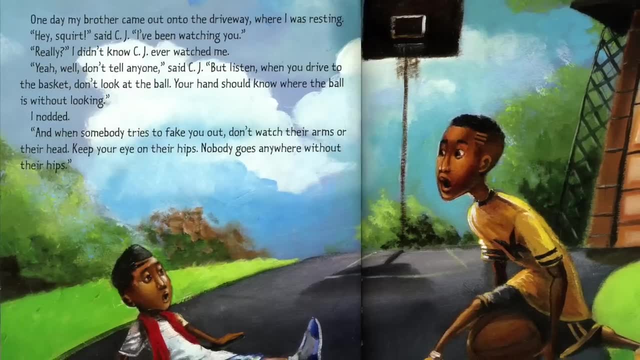 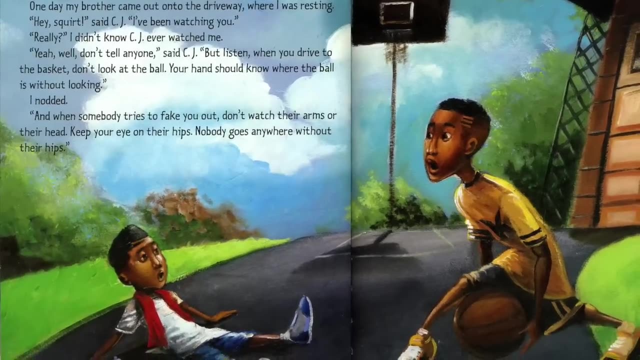 I ran sprints to build up my wind. One day my brother came out onto the driveway where I was resting. Hey squirt, said CJ. I've been watching you. Really I didn't know CJ ever watched me. Yeah well, don't tell anyone, said CJ. 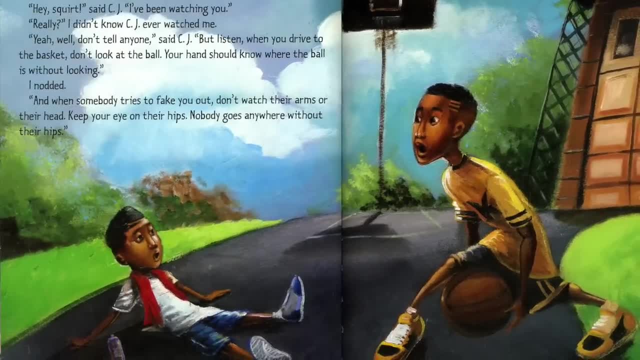 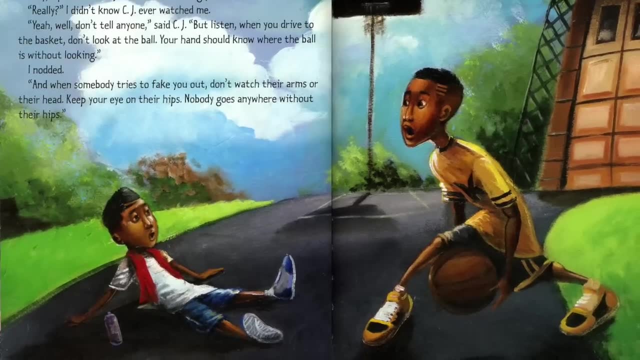 But listen. When you drive to the basket, don't look at the ball. Your hand should know where the ball is without looking. I nodded. And when somebody tries to fake you out, don't watch their arms or their head. Keep your eye on their hips. 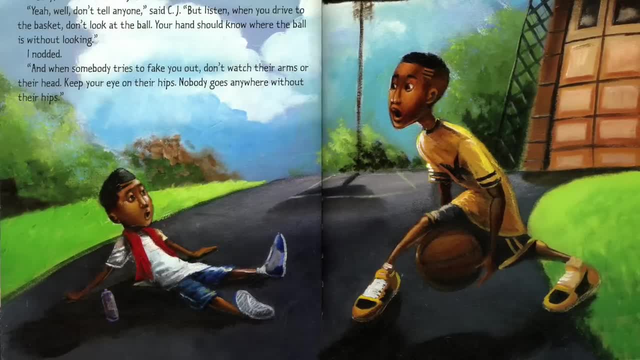 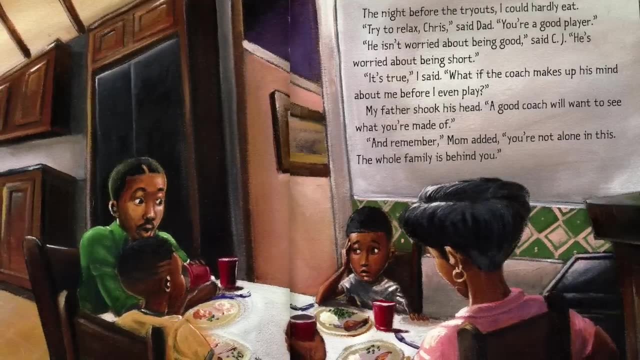 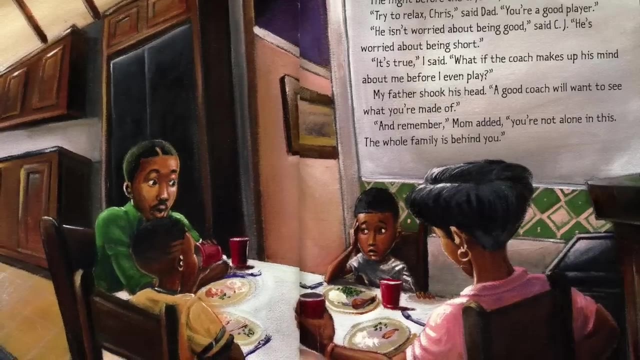 Nobody goes anywhere without their hips. The night before the tryouts I could hardly eat. Try to relax. Chris said: Dad, You're a good boy, You're a good player. He isn't worried about being good, said CJ. 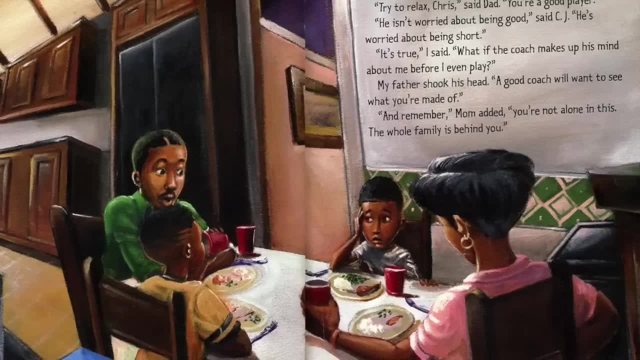 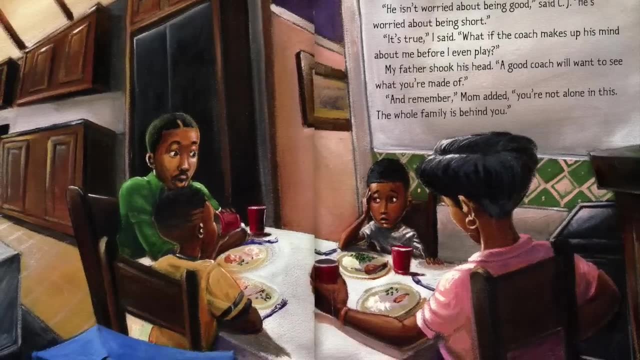 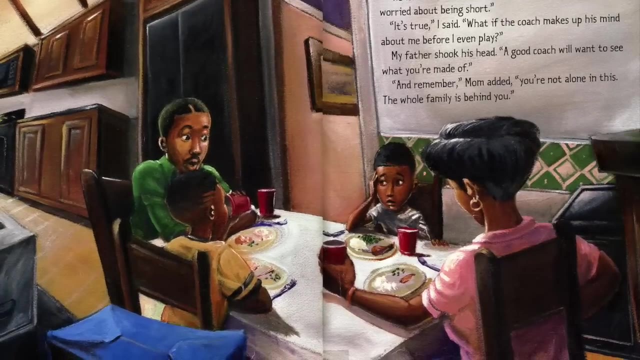 He's worried about being short. It's true. I said: What if the coach makes up his mind about me before I even play? My father shook his head. A good coach will want to see what you're made of And remember. Mom added: you're not alone in this. 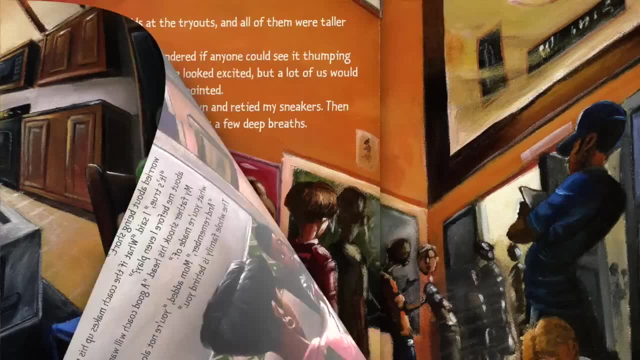 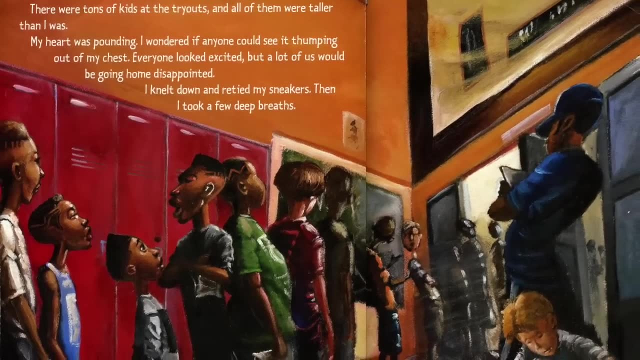 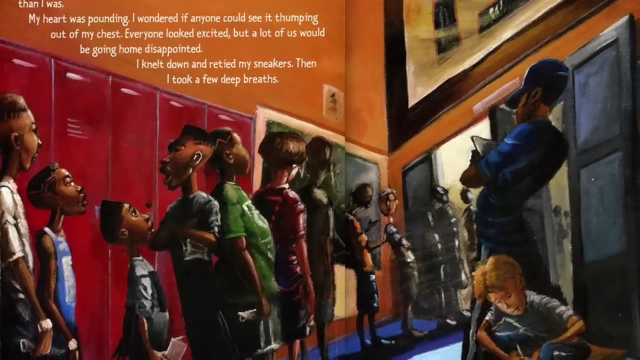 The whole family is behind you. There were tons of kids at the tryouts And all of them were taller than I was. My heart was pounding. I wondered if anyone could see it thumping out of my chest. Everyone looked excited, But a lot of us would be going home disappointed. 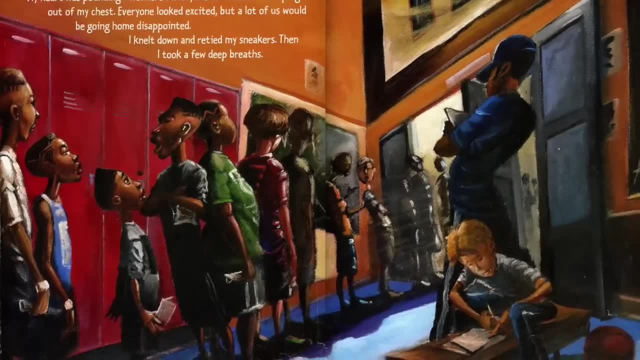 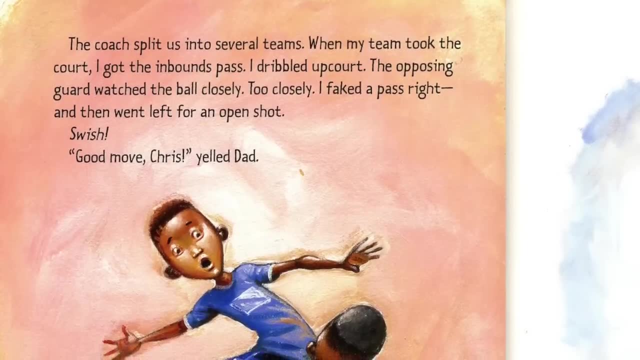 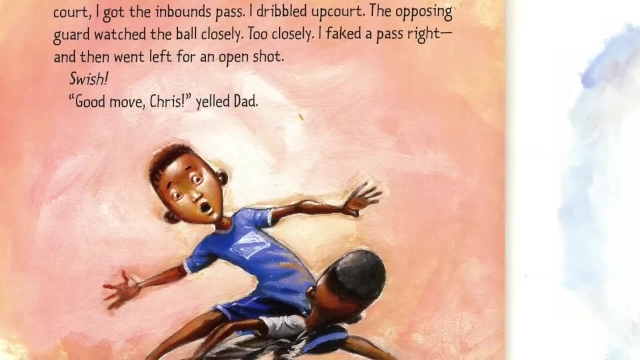 I knelt down and retied my sneakers. Then I took a few deep breaths. The coach split us up into several teams. When my team took the court, I got the inbounds pass. I dribbled up court. The opposing guard watched the ball closely. 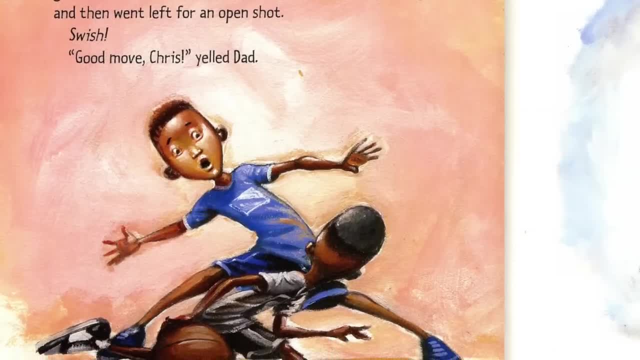 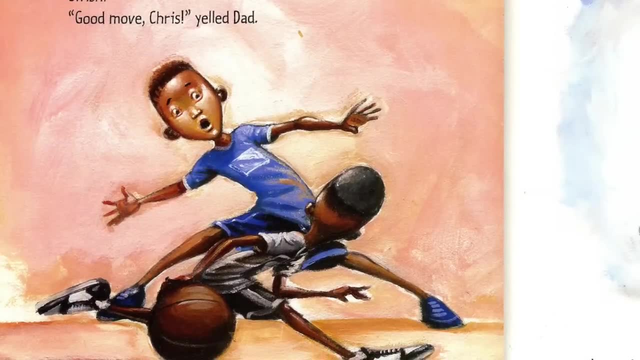 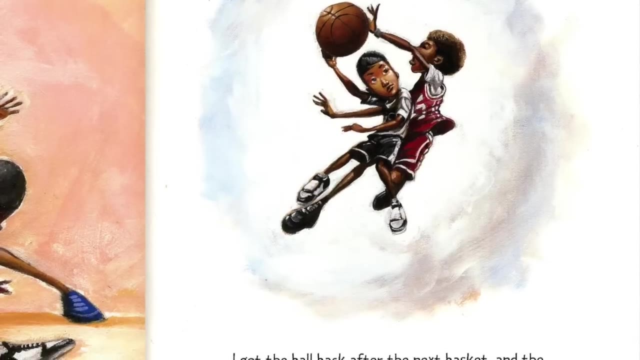 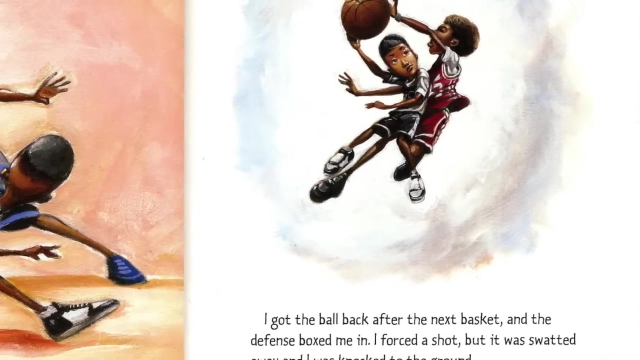 Too closely. I faked a pass right and then went left for an open shot. Swish, Good move, Chris. yelled Dad. I got the ball back after the next basket And the defense. the defense boxed me in. I forced a shot. 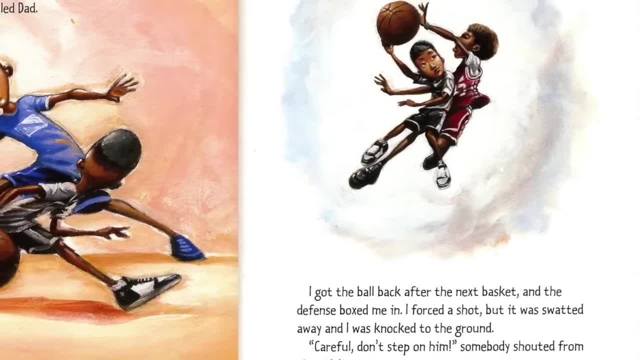 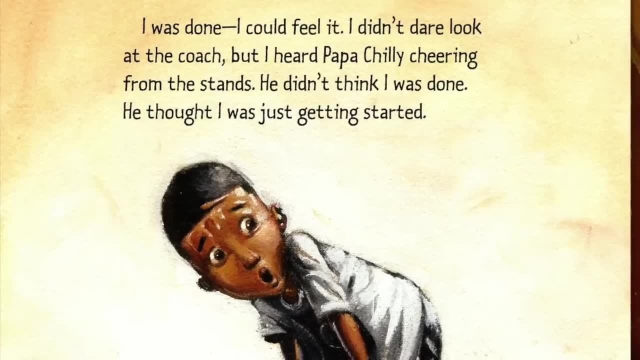 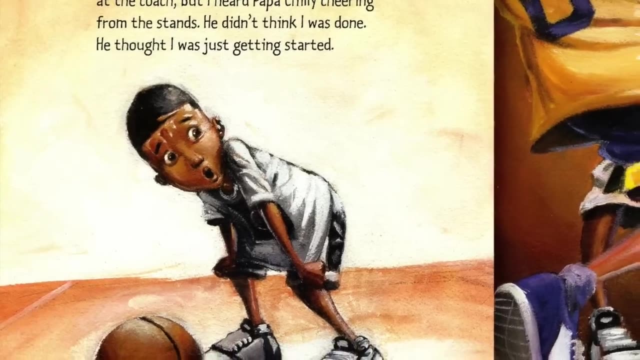 but it was swatted away and I was knocked to the ground. Careful, don't step on him. somebody shouted from the sidelines: I was done, I could feel it. I didn't dare look at the coach, But I heard Papa Chili cheering from the stands. 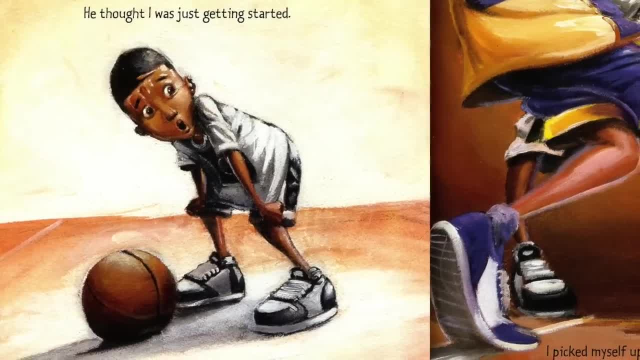 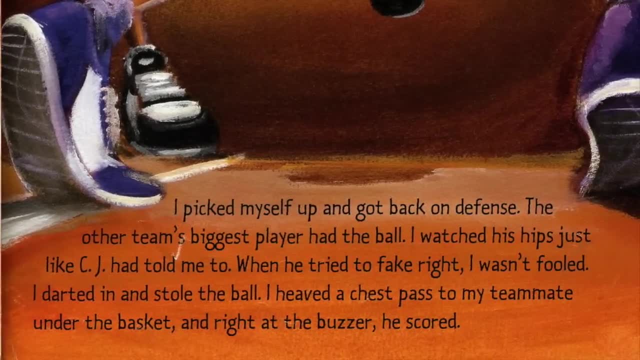 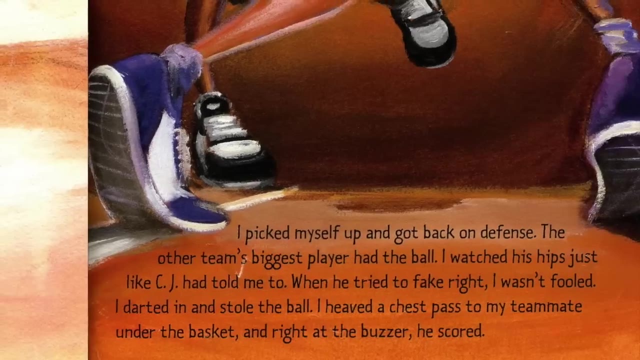 He didn't think I was done. He thought I was just getting started. I picked myself up and got back on defense. The other team's biggest player had the ball. I washed his hips, just like CJ had told me to, When he tried to fake right. 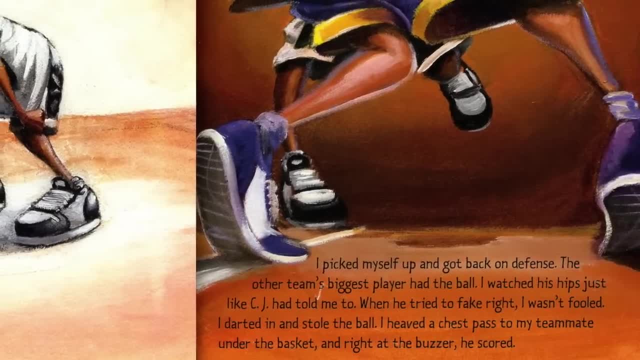 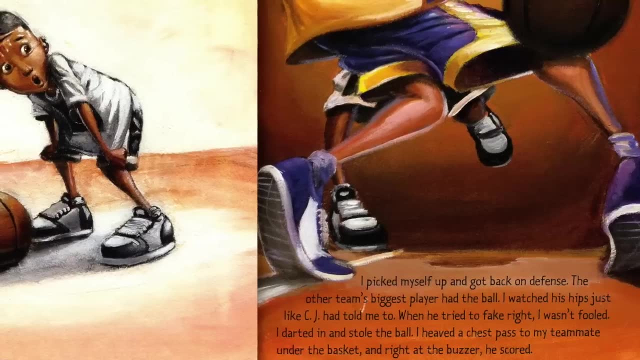 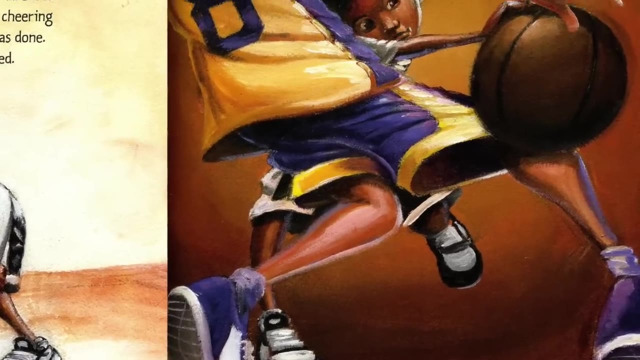 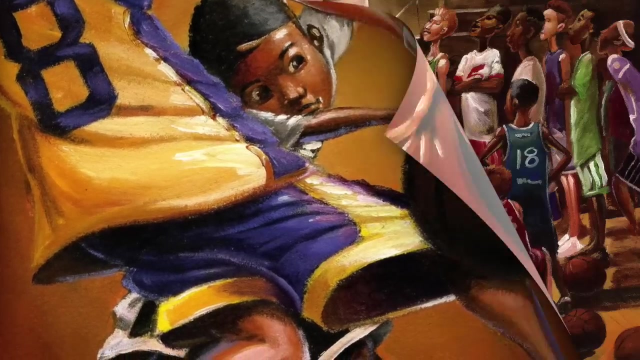 I wasn't fooled. I darted in and stole the ball. I heaved a chest, pass to my teammate under the basket And right at the buzzer he scored. And that was un representa. Afterward we all waited for the big decision. 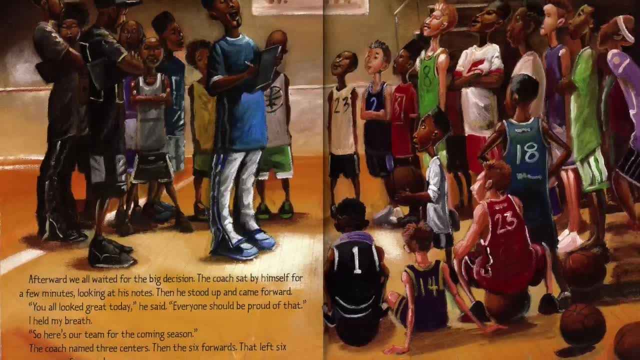 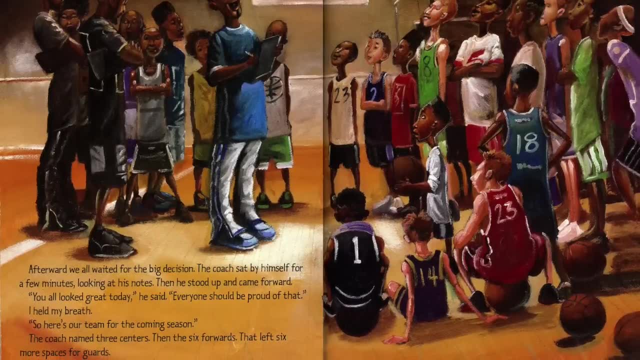 The coach sat by himself for a few minutes looking at his notes. Then he stood up and came forward. You all looked great today, he said. Everyone should be proud of that. I held my breath, So here's our team for the coming season. 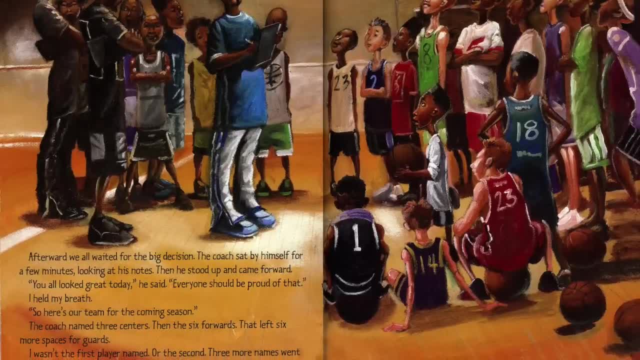 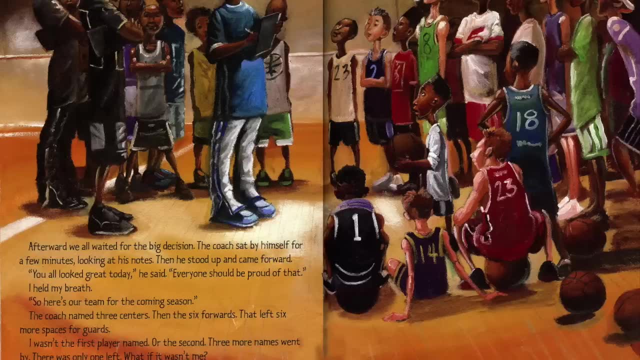 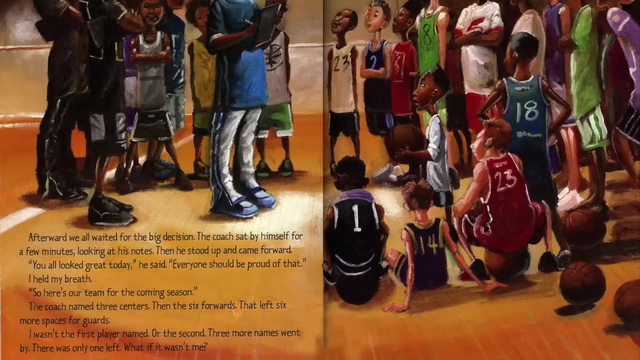 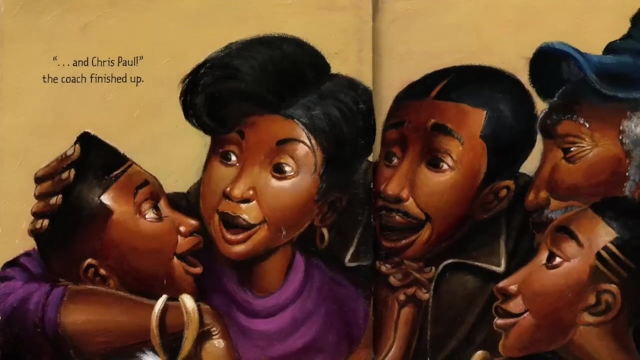 I prepared for the excellent start coming season. the coach named three centers, then the six forwards. that left six more spaces for guards. I wasn't the first player named or the second. three more names went by. there was only one left. what if it wasn't me and Chris Paul? 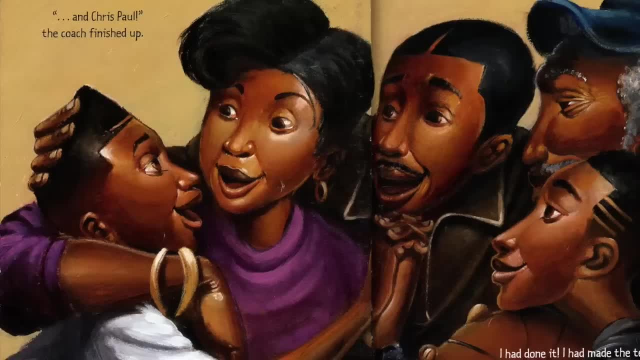 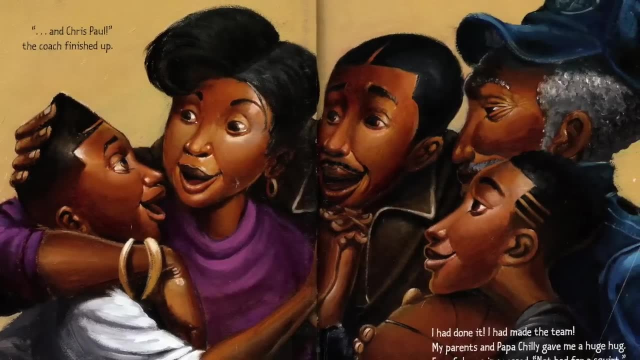 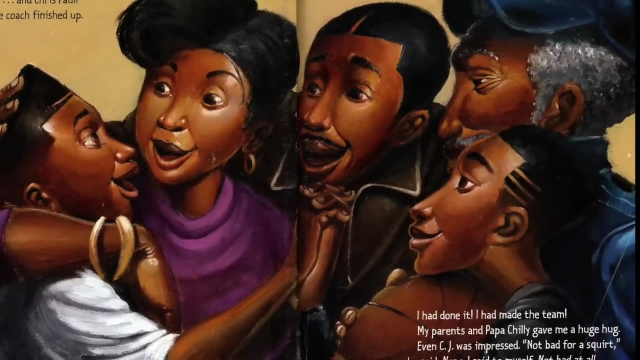 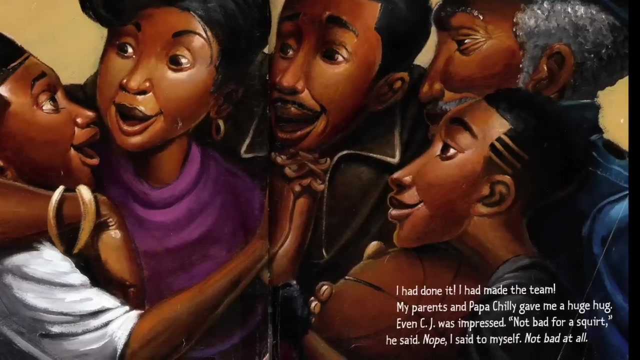 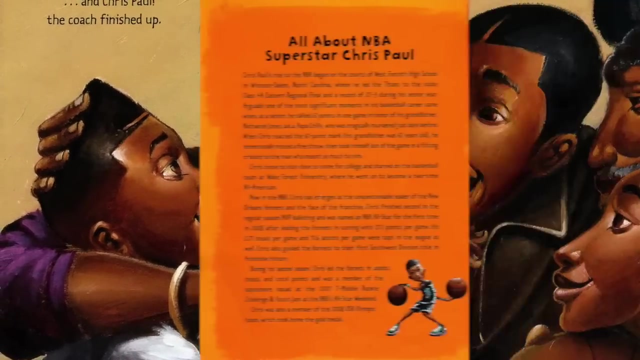 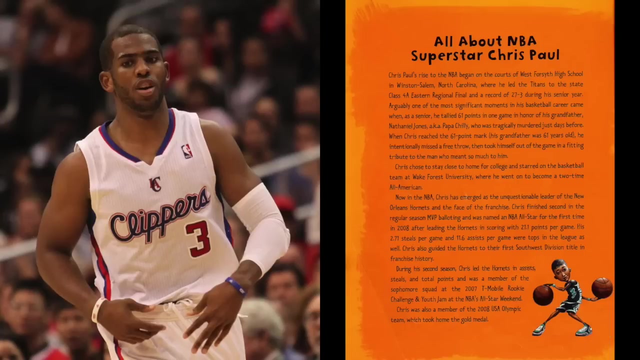 the coach finished up, I had done it, I had made the team. my parents and Papa chili gave me a huge hug. even CJ was impressed. not bad for a squirt. he said nope. I said to myself: not bad at all. all about NBA superstar Chris Paul. Chris Paul's rise to the NBA began on the 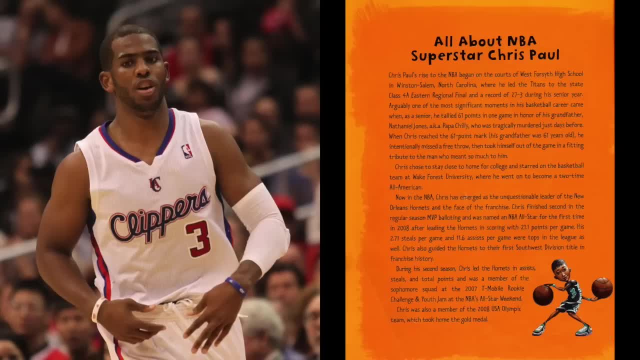 courts of West fourth high school in Winston-Salem, North Carolina, where he led the Titans to the state class 4a Eastern Regional Final and a record of 27: 3 during his senior year. arguably one of the most significant moments in his basketball career came when, as a senior in the NBA, he won the NBA championship. 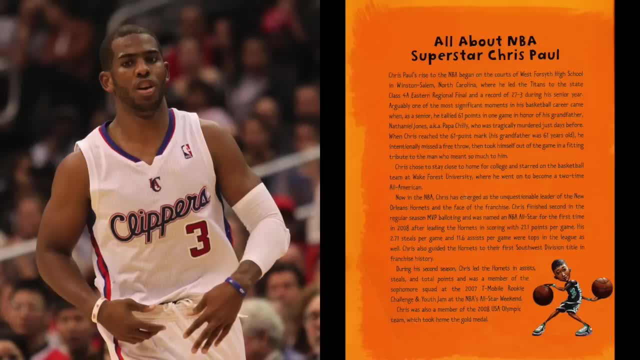 he tallied 61 points in one game in honor of his grandfather, Nathaniel Jones, also known as Papa chili, who was tragically murdered just days before when Chris reached the 61 point mark. his grandfather was 61 years old. he intentionally missed a free throw, then took himself out of the game in a 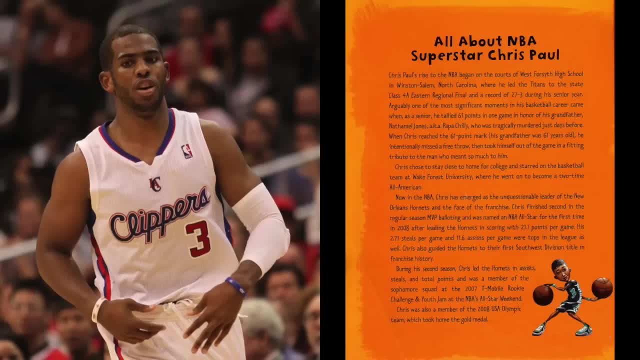 fitting tribute to the man who meant so much to him. Chris chose to stay close to home for college and start on the basketball team at Wake Forest University, where he went on to become a two-time all-american. now, in the NBA, Chris has emerged as the unquestionable leader of 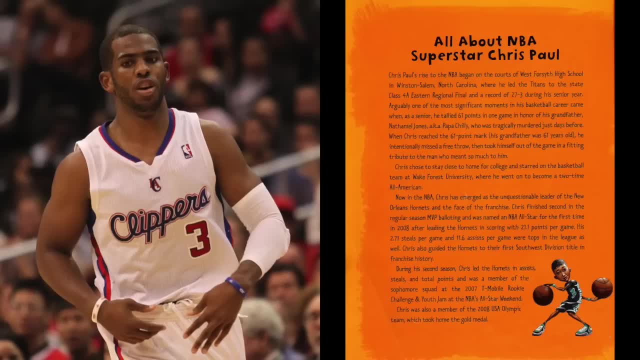 the New Orleans Hornets and the face of the franchise. Chris finished second in the regular season MVP balloting and was named an NBA All-Star for the first time in 2008, after leading the Hornets in scoring with 21.1 points per game- his two